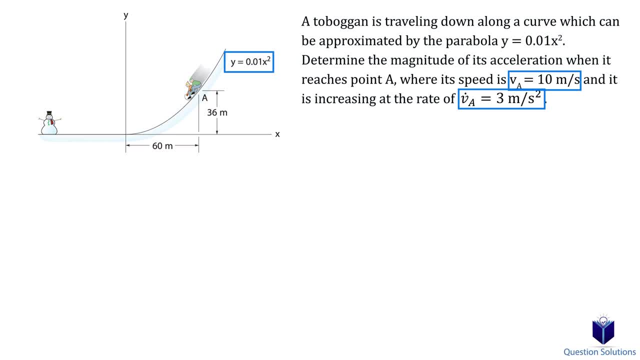 or one derivative of velocity, which again is acceleration. Now, since an equation for the curve is given, we instantly know we need to figure out the radius using the radius of curvature equation. That equation requires three things: the first derivative, the second derivative and the value. 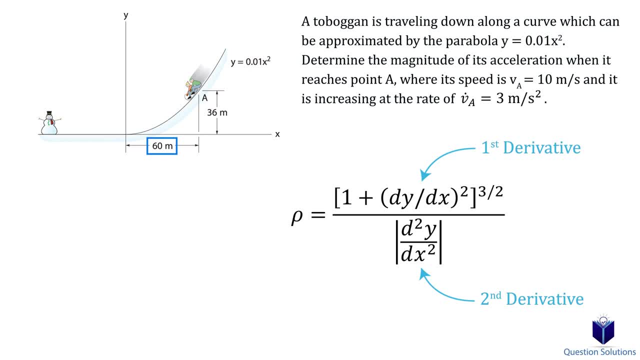 of x at the location where we are trying to find the radius In this question. you can see that it's at x equals 60 meters. So let's do the first derivative of this equation. Now we can do the second derivative. Since we found both derivatives, we can plug it into our radius of curvature. 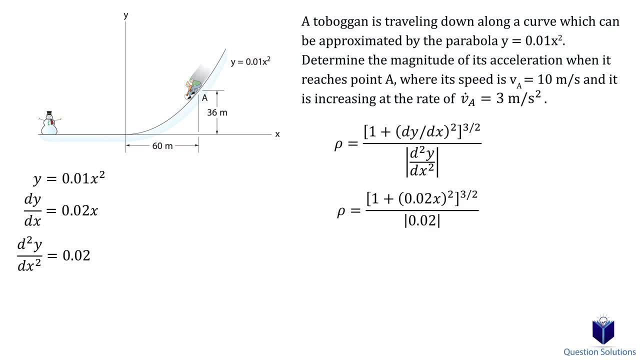 equation To find the radius at x equals 60 meters. all we need to do is substitute that value into this equation. Solving gives us the radius of curvature. Now we can apply the second equation we talked about to find normal acceleration. We know the velocity from the question, which is 10 meters per second, and we just found the radius. 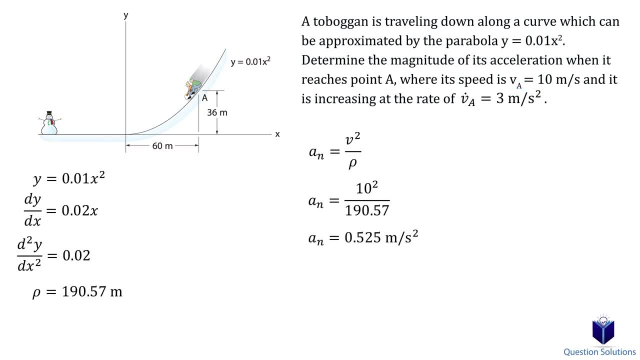 Let's plug them in and solve, which gives us the normal acceleration. Something to remember is that normal acceleration always points towards the center of the curve, while the tangential acceleration points along the tangent, at the point. The tangential acceleration is also given to us in the question, which is 3 meters per second. 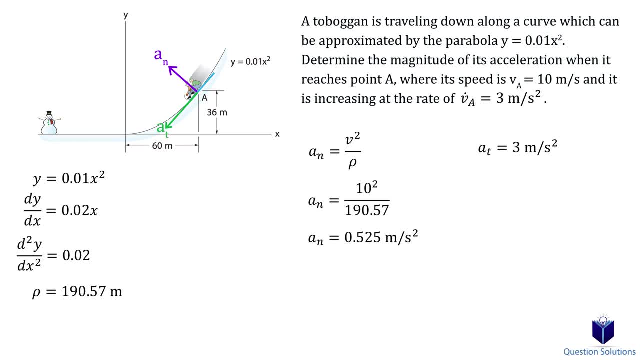 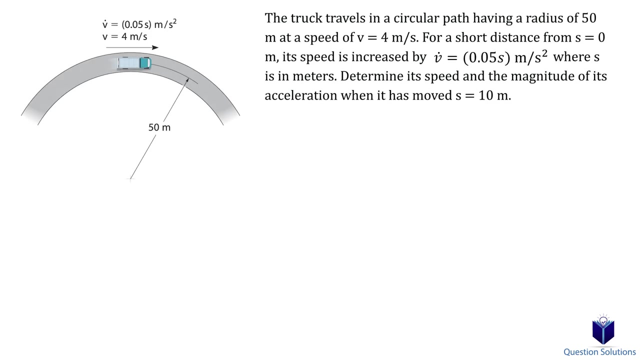 squared. So now we have both accelerations required to find the magnitude. Now we can use the dokładği to find the steepest slope of the energy promo SA だ Modi test. You can substitute that value in case you even want to find the speed of the truck. we want that. 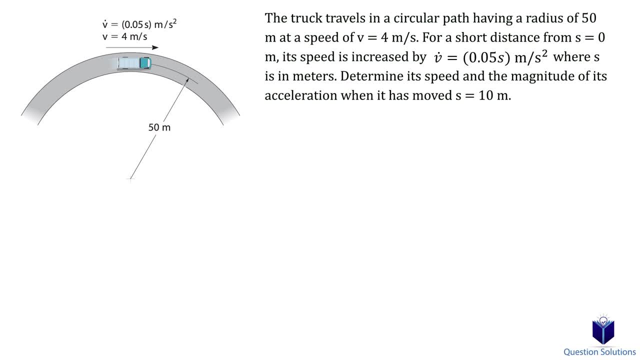 the speed of the truck and the magnitude of acceleration when it moved 10 meters. You can see that we are already given the radius, so we don't need to use the radius of curvature equation. We are also given the velocity, at s equals 0, and the acceleration. 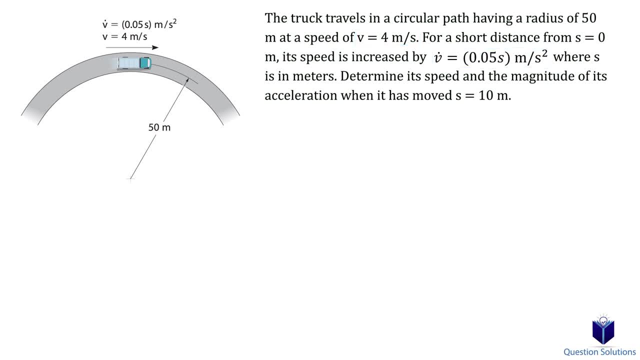 with respect to distance. So let's think about the problem. To find the normal acceleration, we know we have to use our normal acceleration equation, which means we need the velocity when the truck travels 10 meters. So that's what we need to find. first, We can use an old equation. 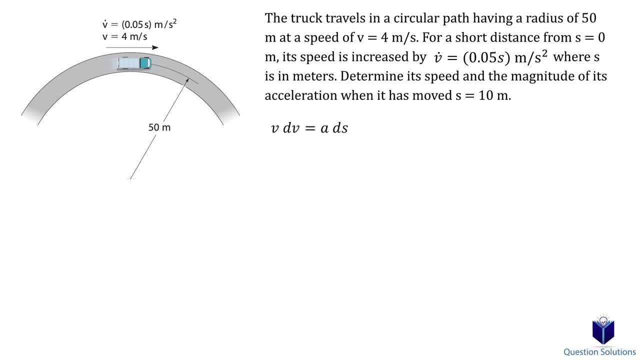 relating velocity and acceleration. to find it, Vdv is equal to ads. Taking the integral of this equation would give us an equation for velocity. So we need to think about the lower and upper bounds of the integral. The velocity starts from 4 meters per second and the distance starts from 0 meters to 10 meters. So this is what. 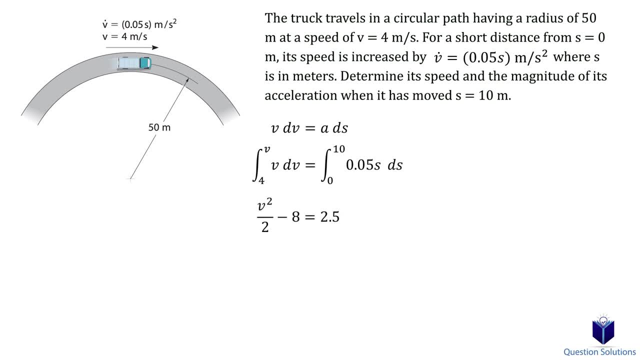 our integral looks like. Solving gives us an equation where we can solve for velocity. Solving gives us the velocity of the truck when it moved 10 meters. Now it's the same. It's just a simple matter of plugging in the velocity and radius into our normal acceleration. 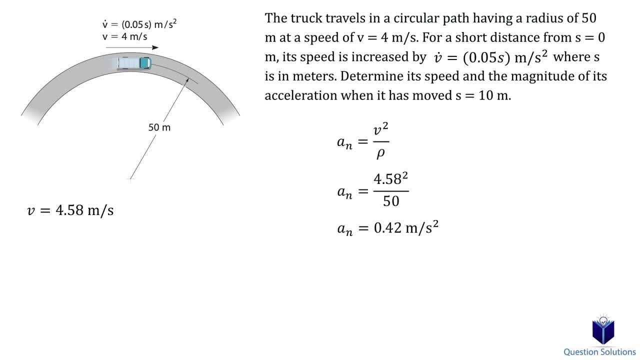 equation Let's solve. to get our normal acceleration, The tangential acceleration also needs to be found. It's actually given to us in the question. All we need to do is substitute 10 meters to figure it out. So let's do that which gives us our tangential acceleration. 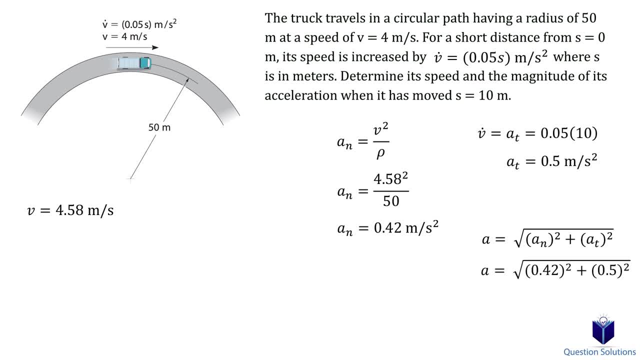 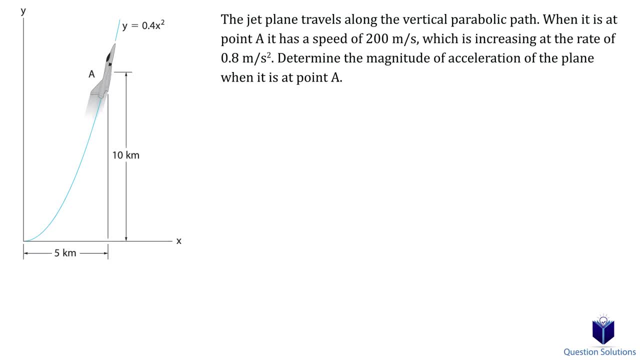 The magnitude can be found using this equation. Solving gives us the magnitude of acceleration. Let's look at one last example In this problem. it's asking us to find the magnitude of acceleration when the jet is at point A. Looking at the diagram, we see that the curve is represented with an equation. 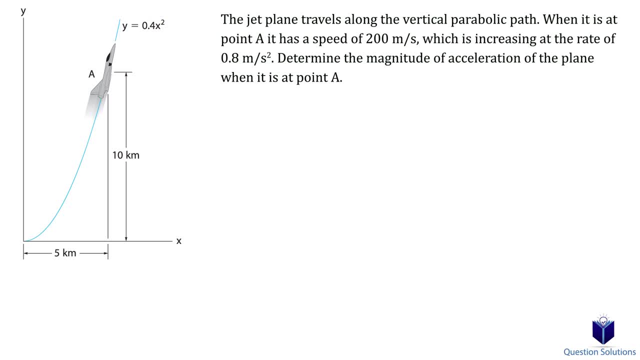 So the first thing we have to do is take the first and second derivative of the equation. Let's start off with the first derivative, Now the second derivative, Now we can plug them into our radius of curvature equation. Looking at the diagram, we see that the x value at point A is 5 kilometers, So let's substitute that into our equation. 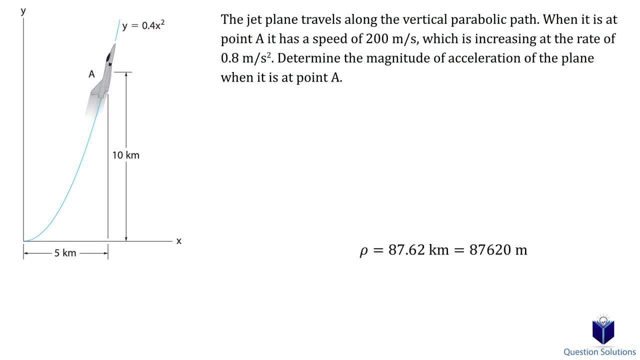 Now we can find the normal acceleration. The velocity is given in the question, which is 200 meters per second, and we just found the radius, So let's plug it in and solve. The tangential acceleration is also given to us in the question: It's 0.8 meters per second squared. 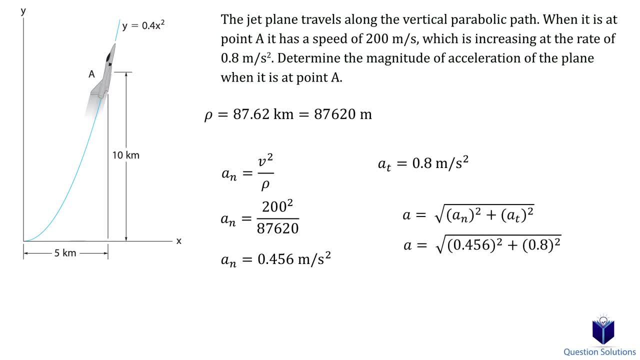 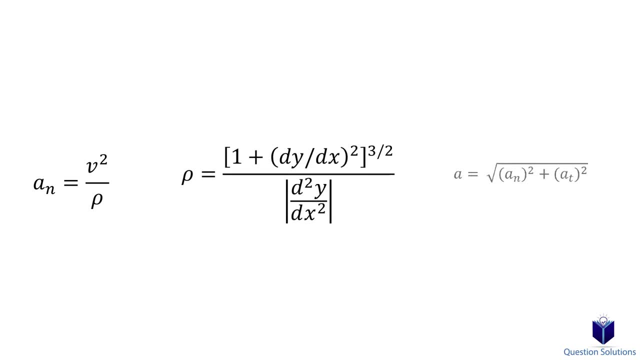 To find the magnitude. we just need to use our magnitude equation and solving gives us our answer. Most, if not all, questions in this chapter rely on three new equations I showed at the beginning of this video. There will be some questions where trigonometry will be very useful. 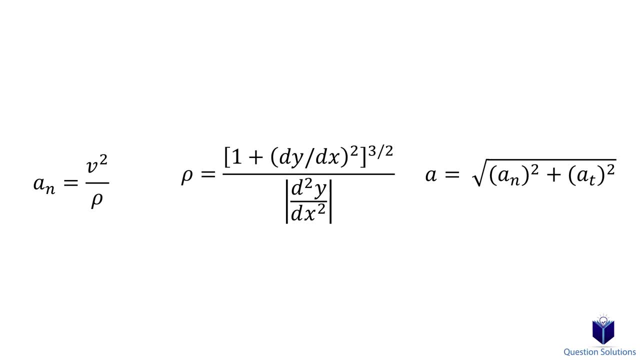 but the core of the problems still rely on the three new equations you have to use. I listed some other solved questions that might be challenging in the description below. Thanks so much for watching and I hope this helped. Best of luck with your studies.